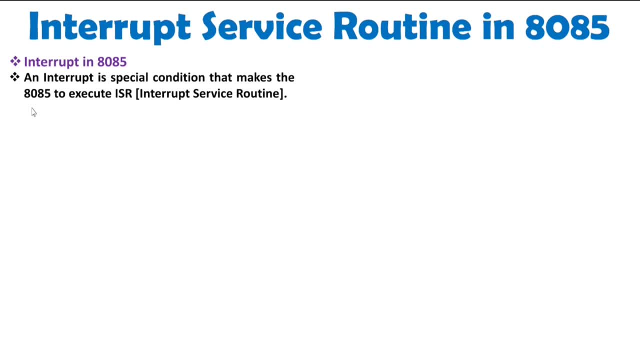 interrupt. it is a special condition that makes microprocessor 8085 to execute ISR interrupt service routine. Microprocessor checks interrupt during every instruction And once interrupt occurs, microprocessor will first execute current instruction. After that it will push PC on the stack and then it will reset interrupt flag so that no more interrupt. 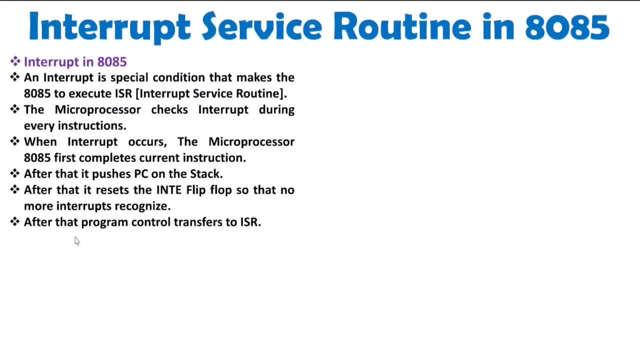 can be recognized And then it will be transferring its program control to ISR and interrupt service routine is getting executed. Let us try to understand that by graphical representation. So here we are having main program while you execute main program, Let us say there is interrupt. 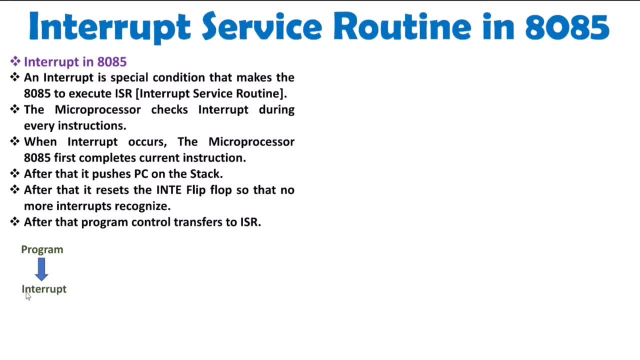 which is occurring in 8085.. So as if interrupt occurs, microprocessor first will have to execute current instruction. After execution of current instructions it needs to transfer control to the interrupt service routine. But before it transfers control to the interrupt service routine, my dear students here, microprocessor will disable. 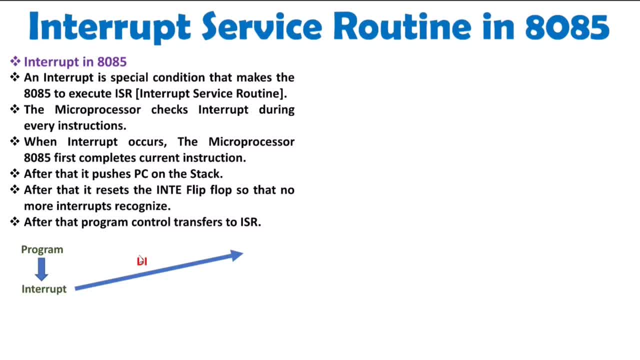 interrupt flag first by DI instruction and this DI instruction that will get executed by microprocessor 8085.. Now here it will push program counter first. Why The reason is it needs to store execution of main program before it transfer controls to the interrupt program. It will have to store location of main program. This is main program, right? So push PC. 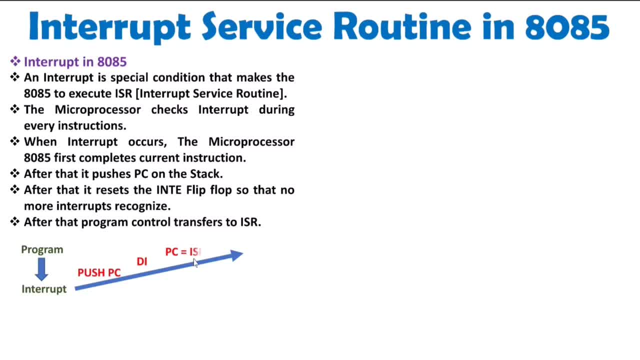 will happen first. After that PC will get transferred to interrupt service routine. So here there will be interrupt service routine program and once it starts to execute interrupt service routine program and at the end it will have to perform return operation. Once it performs return operation it will. 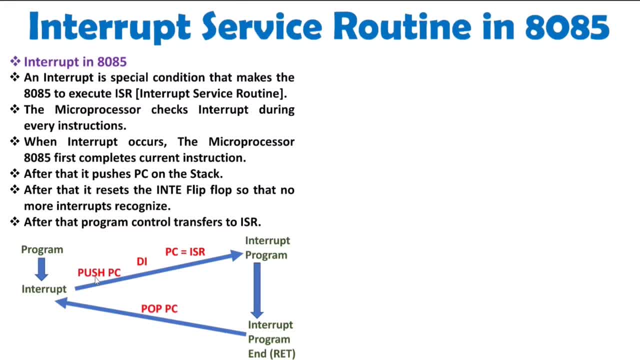 be performing POP PC operation. Why? The reason is push PC is having original data of this address over here on stack, So to retrieve that data we need to have POP PC operation. Once it performs POP PC operation, program counter will be available here and it will. 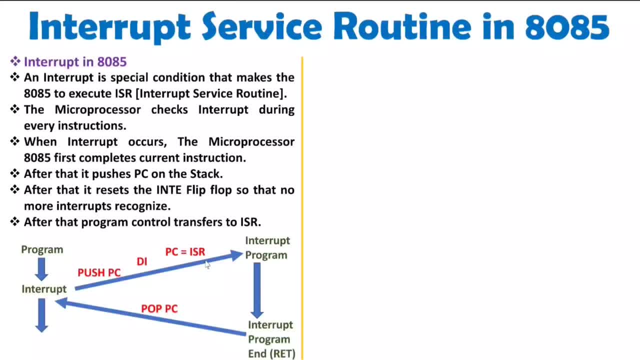 execute main program. So this is the complete process which is happening, But here there are few steps that we need to understand so that I will be explaining you all those things by steps over here. So, my dear students, interrupt steps in 8085 is having two instructions, which is very essential. One is EI instruction, that is, enabling interrupt. 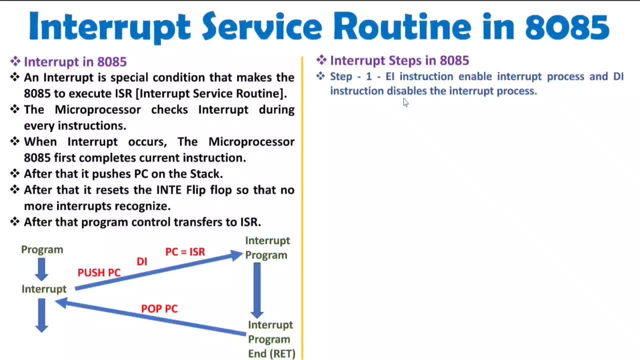 process. and second is DI instruction that is disabling interrupt process. Now remember, See DI instruction that we don't execute as per programmer, but EI instruction that is very essential that has been executed by programmer during interrupt service routine. So EI instruction that has been 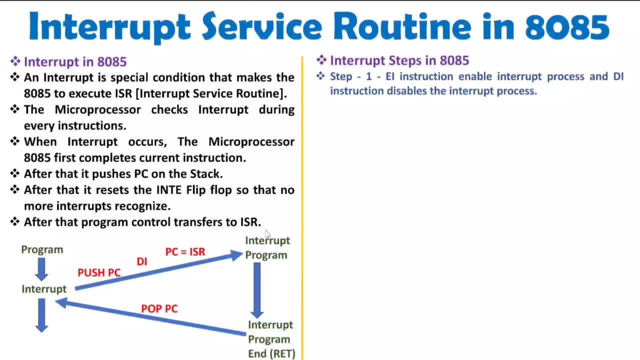 written by programmer during the program of interrupt. Now in second step we need to see what has been done by 8085.. 8085. So as if you execute main program, at that time microprocessor will be checking continuously INTR line, that is, interrupt request line right, and if INTR goes high then you can say interrupt. 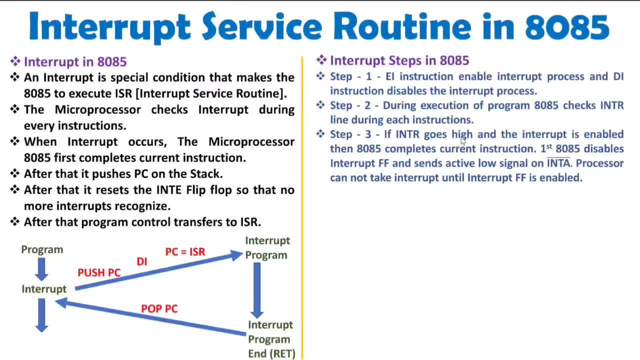 is arised over here. So what will happen when INTR goes high? the interrupt is enabled, then 8085 will execute current instruction first. So whenever interrupt comes, microprocessor will have to execute current instruction. It cannot execute interrupt directly. it will have to execute. 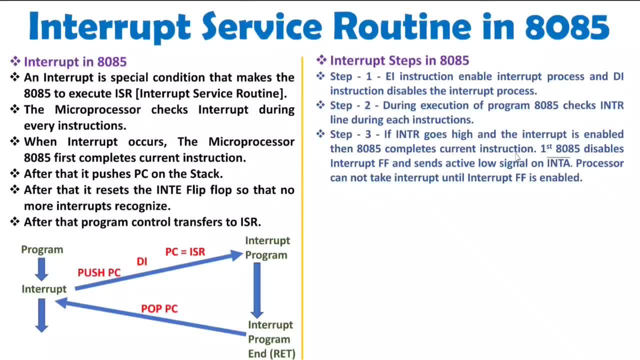 current instruction. Once it executes current instruction, first it will disable interrupt flag and that will be done by 8085.. We are not doing it as a programmer. we don't perform this right. that is been performed by 8085.. And as interrupt flag is disabled, microprocessor cannot receive another interrupt. Remember. 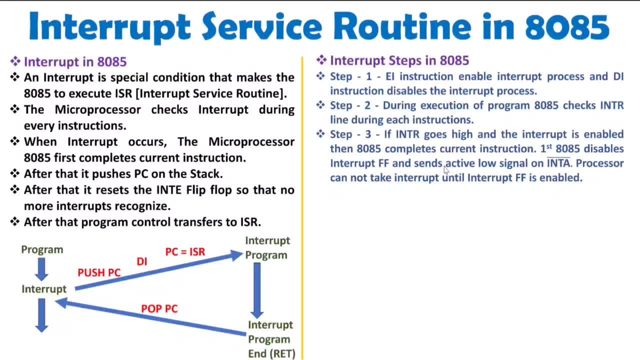 this: After that, INTA bar signal that will be given to external hardware. This signal will be given to the hardware which is giving interrupt to microprocessor right, and processor cannot take interrupt until interrupt flag is enabled. Now, my dear students, in next step, microprocessor will give INTA bar active low signal to external. 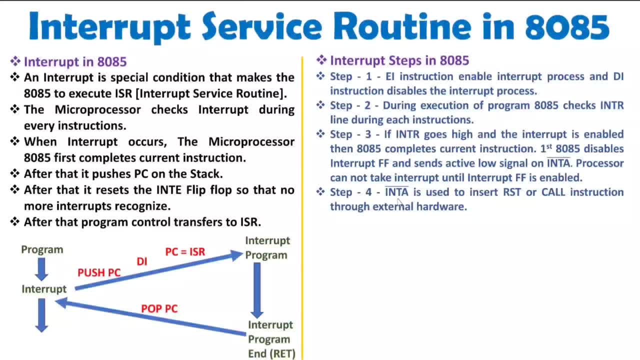 device and this signal is provided to external device for inserting RST or call instruction. this RST instruction that is been used for interrupt service, as well as external devices, can send call instruction also. With RST instruction, External needs to fetch only one byte to the microprocessor, but for call instruction, external device will have. 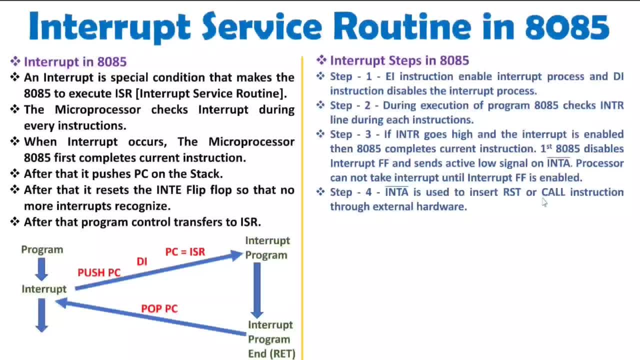 to give three bytes for given transfer control. So microprocessor will receive RST or call instruction during INTA bar signal and that is what microprocessor is giving. INTA bar is been given by microprocessor, INTR that will be given by external device right Now in next step once. 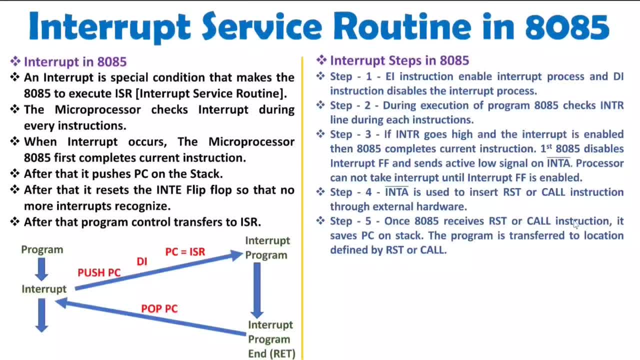 RST or call is been received, microprocessor will have to save its current location of program counter on stack. So you see when interrupt is coming, microprocessor will have to push program counter on the stack right After that program is transferred to the location defined by RST. 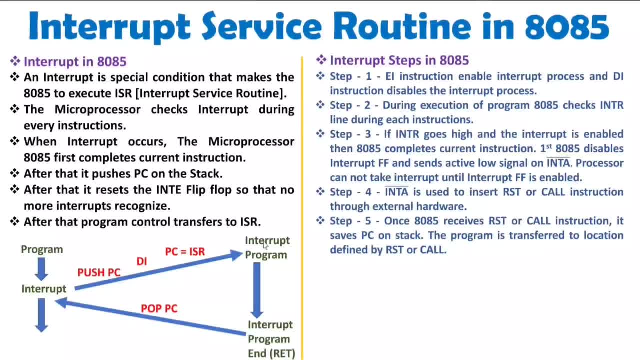 So it will get transferred over here, right? It may be as per RST instruction or it may be as per call instruction. After that program on RST or call is referred as interrupt service routine, that will get executed by microprocessor, and during that execution of program microprocessor will have to 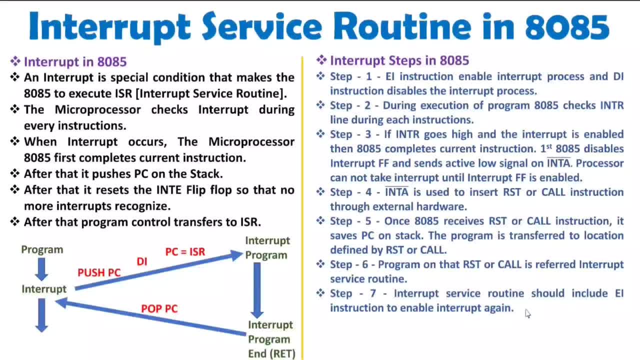 include EI instruction to enable interrupt again. So so, so, so, so so this execution of interrupt program microprocessor will have to write ei instruction so that microprocessor can receive another interrupt and at last there will be ret instruction that is to end subroutine of this interrupt. and when you write ret it will retrieve pc from the stack. 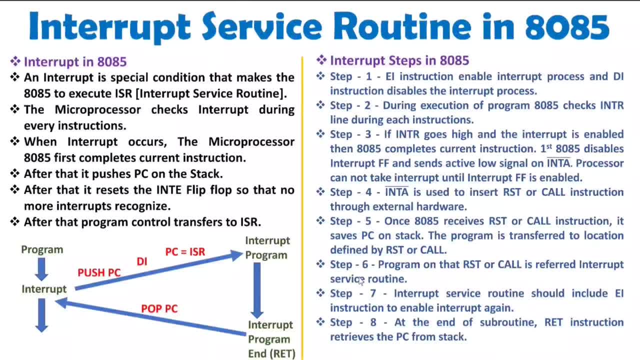 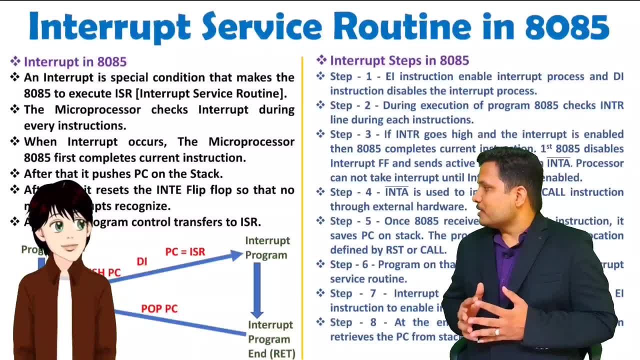 so that is how all the steps are there. with 8085 it is sir. can i ask you one question? i love to reply your question, my dear john. it is. sir, during execution of interrupt service routine, is it possible that we can receive another interrupt and we can provide service to? 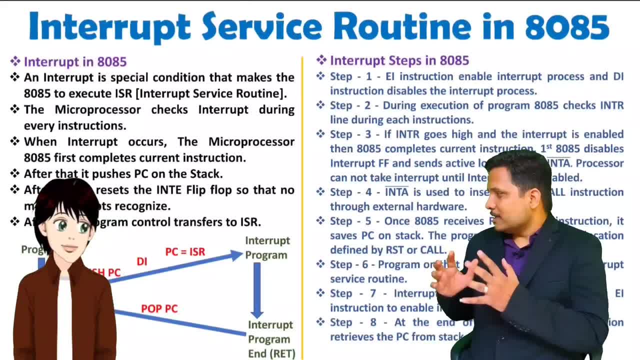 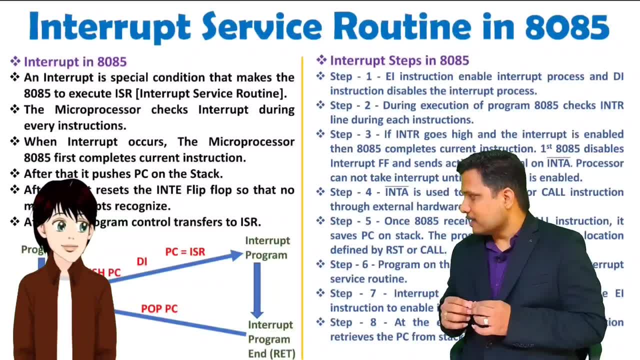 another interrupt during execution of that interrupt. yes, john, this question is quite interesting, but with this question there is no straight forward answer, right? but let me try to explain you what is the answer of your question in this powerpoint presentation. all only my, dear john. as per your question, what i understood is during: 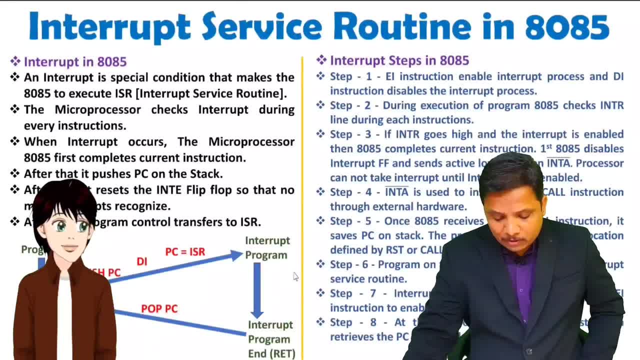 execution of interrupt. is it possible to receive another interrupt? so it is possible, but for that we need to see whether programmer has executed ei instruction in this program or not. like you see, when interup is arising, microprocessor is executing di internally. so now, as di is executed by, 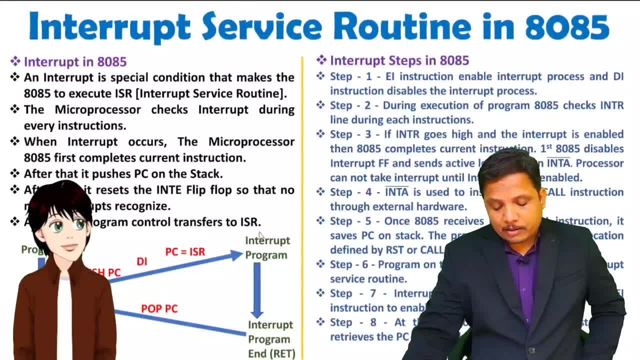 microprocessor we cannot take another interrupt. but during program. if you write ei over here means enable entering up over here, then during rest program execution if interrupt is coming, then we can be able to execute that. but if you write enable interrupt at last of this interrupt program, in that case during interrupt program. 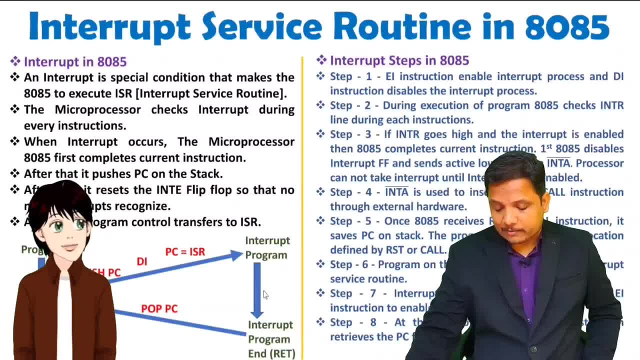 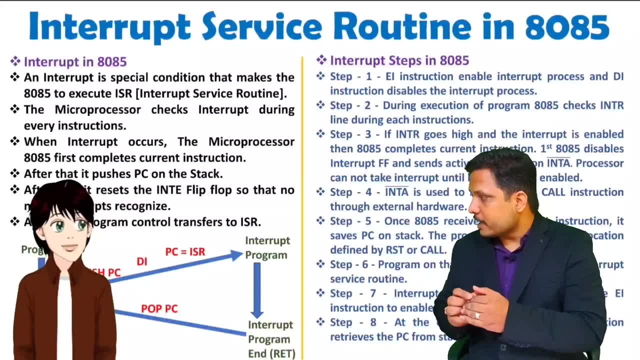 you cannot take another interrupt, right? so, john here, what is happening here? we need to see where to write ei. if you write at initial program of that interrupt service, then during program of interrupt we can be able to take another interrupt. but if you write that, enable interrupt. 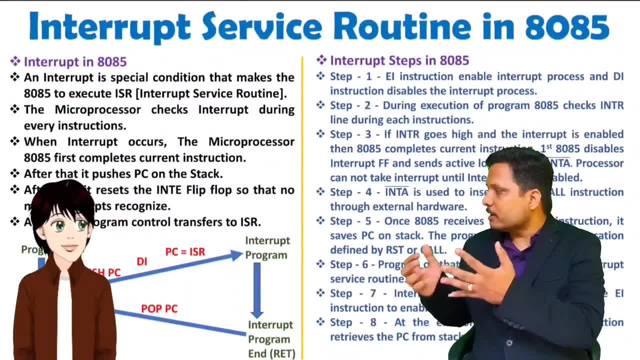 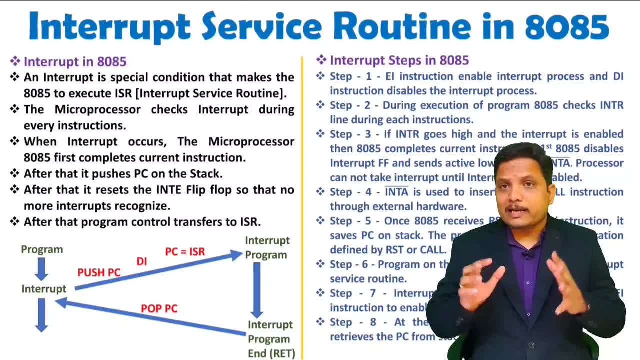 at last. then during execution of interrupt program, we cannot take another interrupt while executing service to current interrupt. so, my dear students, i think now it is clear to you what is interrupt steps, and if you want to give higher priority to whatever interrupt, in that case what you need to do is you will have to write ei at last. 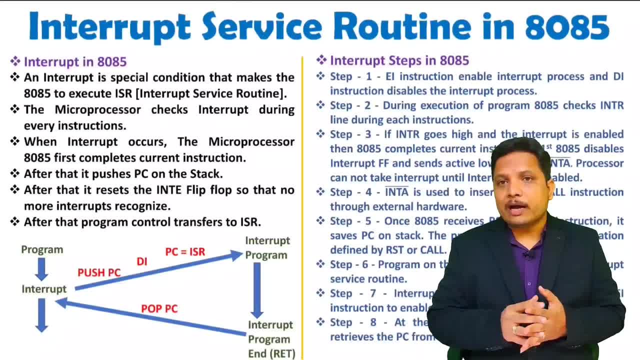 last of that interrupt program. but if you have lower priority of interrupt, in that case you should be writing that at initial instructions of interrupt program. i think it is clear to you now. thank you so much for watching this video.